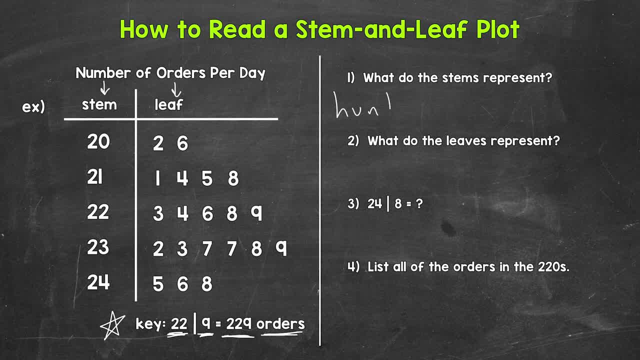 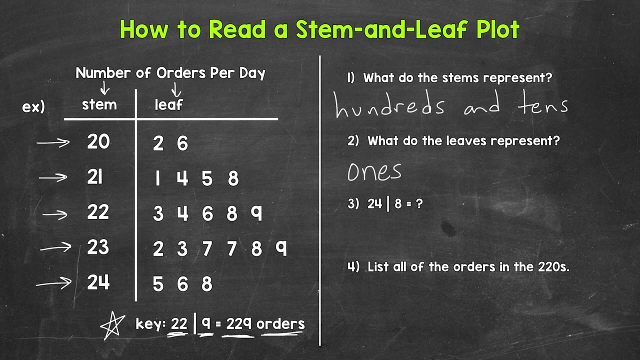 Well, the stems again represent the hundreds place the hundreds digit and the tens place the tens digit. And then the leaves represent the ones place the ones digit. For the stems, we have 20,, 21,, 22,, 23, and 24.. So we have the 200s, the 210s, the 220s, the 230s and the 240s. 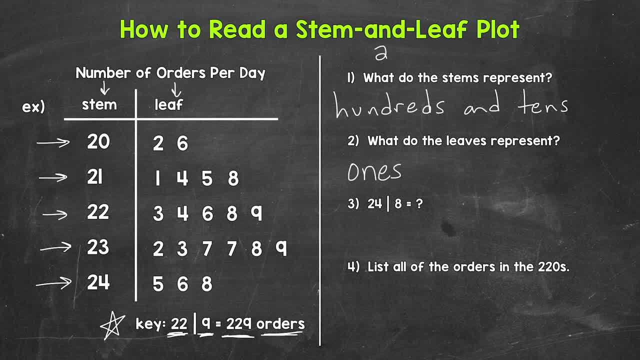 Think of the stems like this: So our first stem of 20, the hundreds place and tens place, and then the leaves will go in the ones place. Then we have the stem of 21,, and then the leaves will go in the ones place. 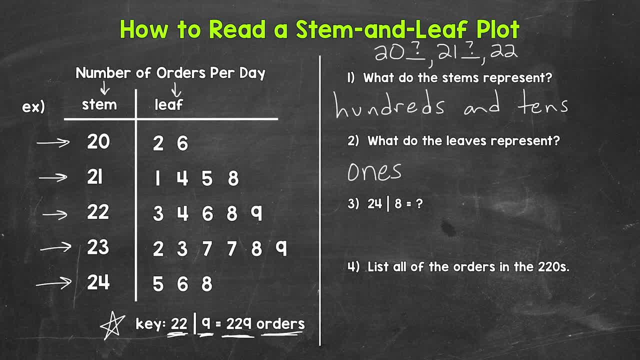 Then we have the stem of 22,, and then the leaves will go in the ones place. Then the stem of 23,. leaves go in the ones place, And then, lastly, the stem of 24, leaves go in the ones place. 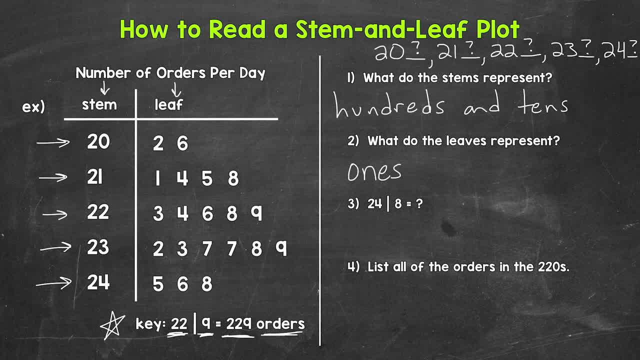 Let's put this all together and look at number three, where we have a stem of 24 and a leaf of 8.. So, looking at the stem and leaf plot, we have a stem of 24, a leaf of 8, so the hundreds. 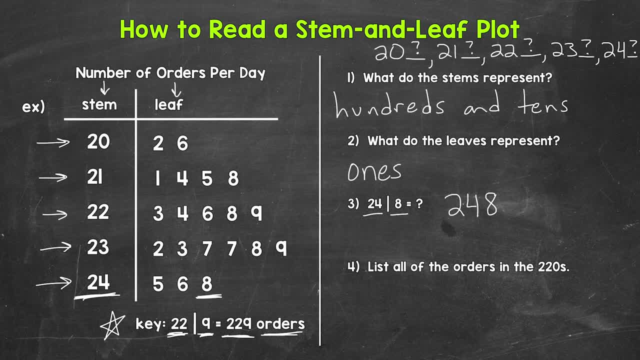 tens and then ones, That gives us 248.. So again, the 24, the hundreds place, the tens place and then the one leaf placed. So we put the stem and the leaf together and we get 248.. And then, lastly, 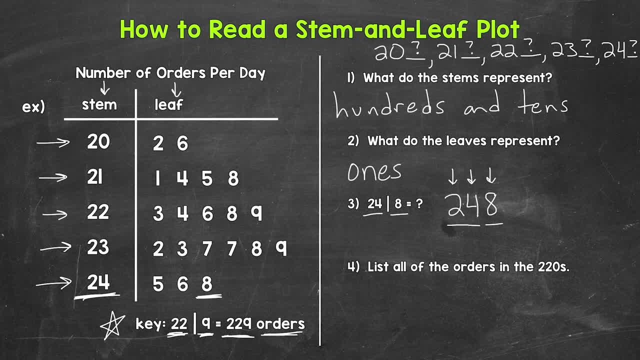 let's move on to number four, where we have list all of the orders in the 220s. Well, we need to look at the stem of 22 and put that together with the leaf of three, the leaf of four, the leaf of.